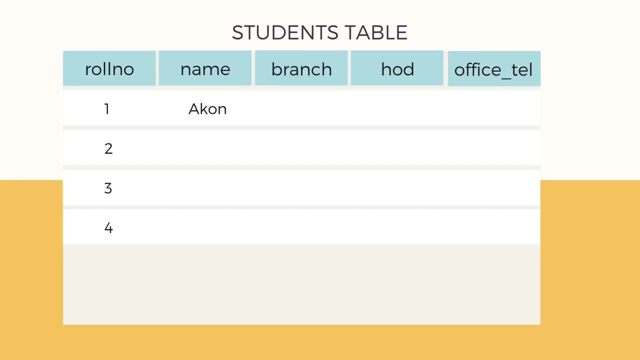 1,, 2,, 3 and 4, put in the student's name, their branch name, the name of the hod and the department telephone number. Now, in this case, the branch name, the hod name and the telephone number are same for all the entries that we make. 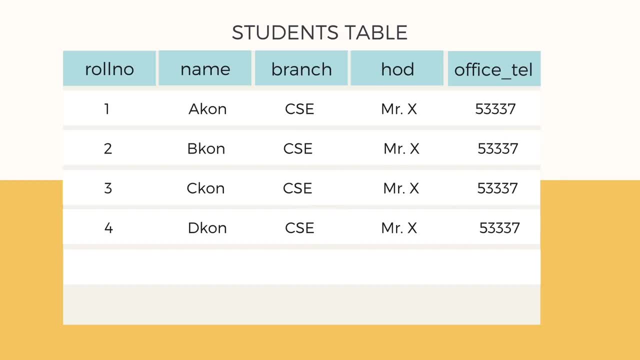 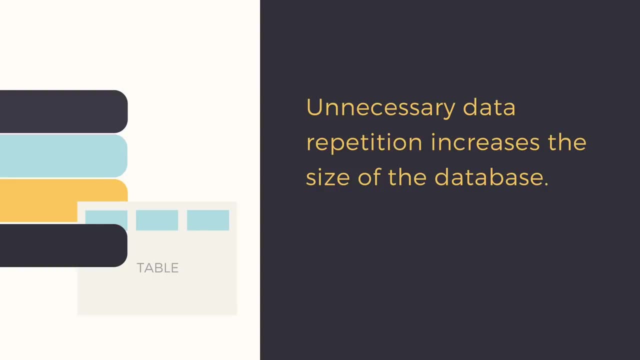 whenever a new student entry is created, this entire information is repeated, and this is what is redundancy. now, this data redundancy not only increase the size of our DB unnecessarily, but it also leads to multiple other issues, like we talked about. so let's see what these issues are. there are. 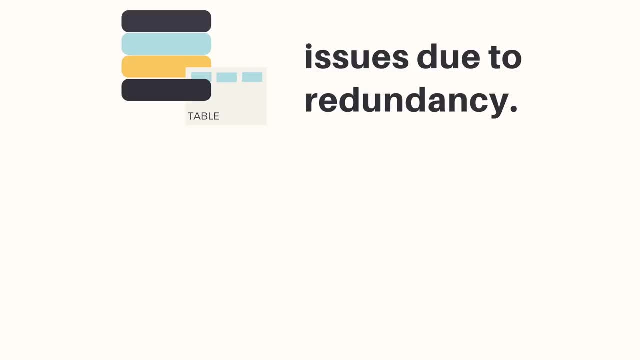 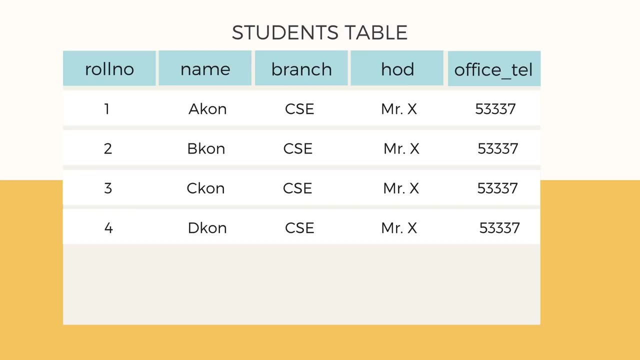 three main problems that data redundancy causes. these are the insertion anomaly, the deletion anomaly and the updation anomaly. so let's start with insertion anomaly. now we already have four students data in our table. if we have to add a fifth student, we will have to repeat the same. 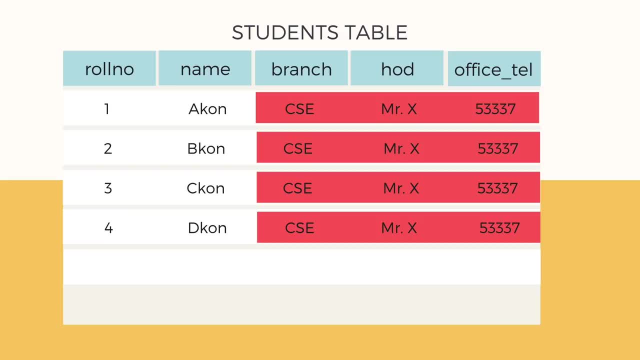 data which holds the branch information, like branch name, the name of the HOD and the branch telephone number. again, we will have to repeat the same data which holds the branch information like: and if we have to enter the data for hundred more students, we have to repeat the data a hundred more. 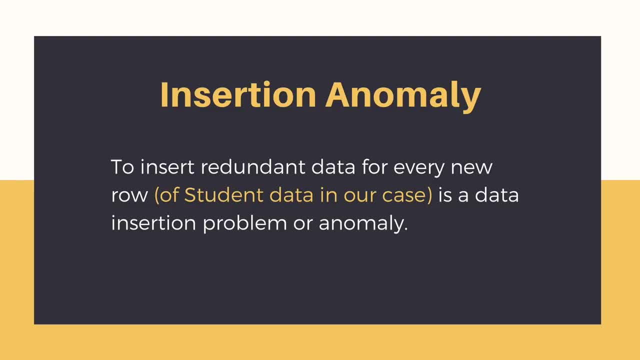 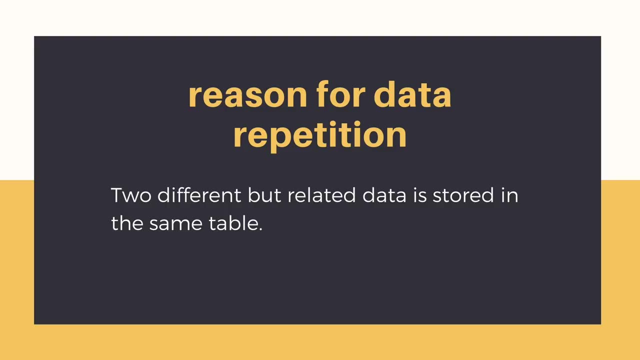 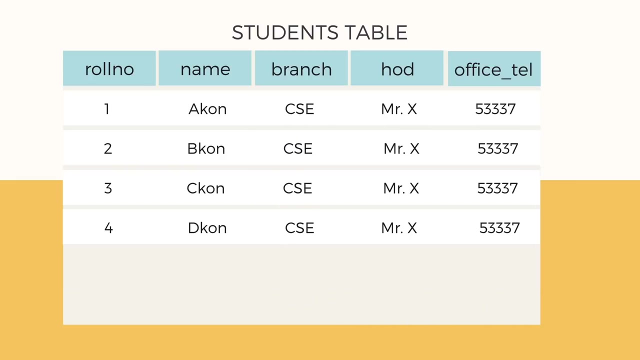 times, which leads to insertion anomaly, because the repetition of data will only increase as we insert more entries to our table. now this repetition arises because in our example, we are unknowingly, unintentionally, saving two pieces of information in every row: student information and branch information information. now, if we start deleting student information, the branch 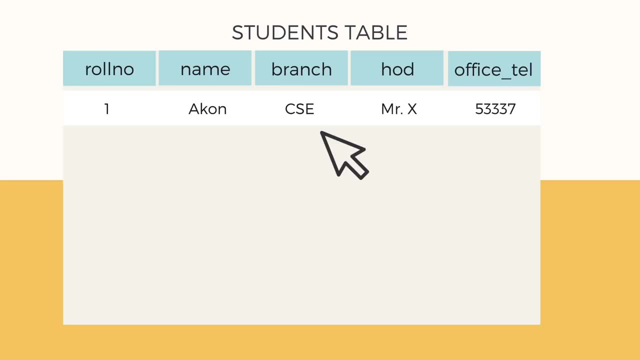 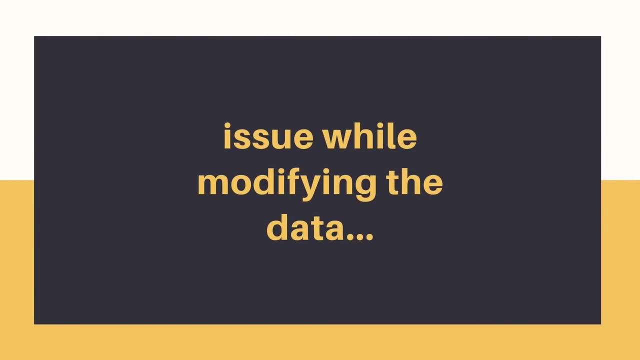 information is also deleted simultaneously, and when we delete the last student row from the student table, we also unintentionally delete the branch information. so now we don't have any student information and we also don't have the branch information because we deleted it, which leads to deletion problems and is also known as deletion anomaly. now let's see what. 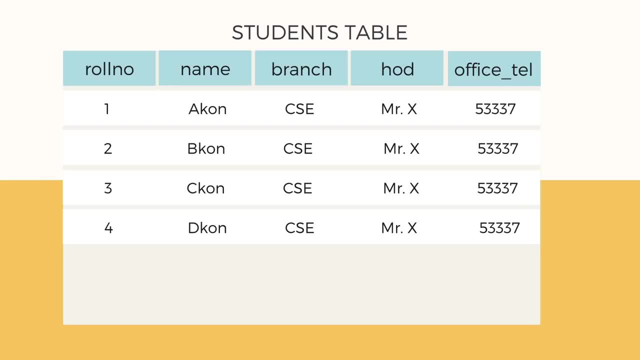 updation anomaly or modification anomaly is. so, let's say, if the HOD or the head of the department leaves for some reason, making the students happy, and the department gets a new HOD and the system administrator has to update all the student records with a new name of the HOD, this is modification anomaly. 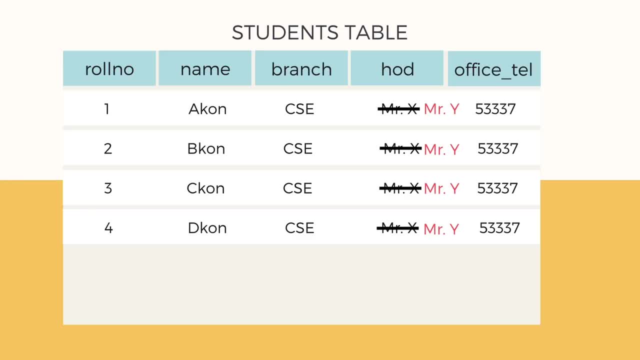 because this is hell lot of a work which the administrator has to do to update every single record with the new HOD name and during modification, if even a single row is missed out, it will lead to inconsistent data. hence, data redundancy can also lead to inconsistency in data as a result of updation anomaly. now you understand that. 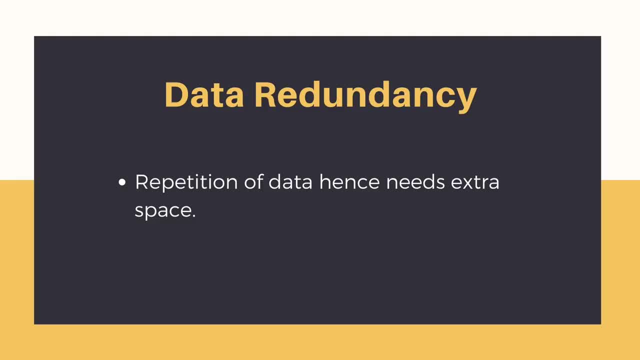 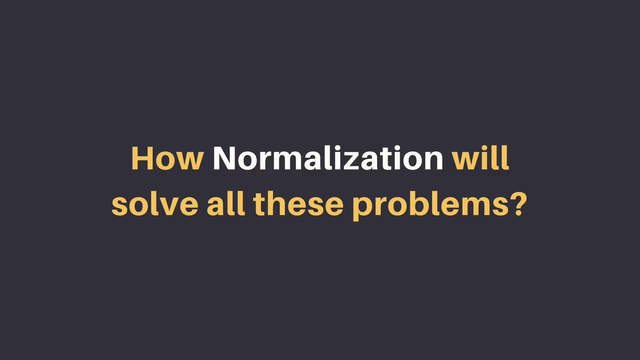 data redundancy is pure evil, not only because it eats up extra space, but it leads to problem in inserting new data, deleting the data and deleting the data a huge problem if we have to update the data. so now the million dollar question is how normalization will solve this problem. so normalization will break the 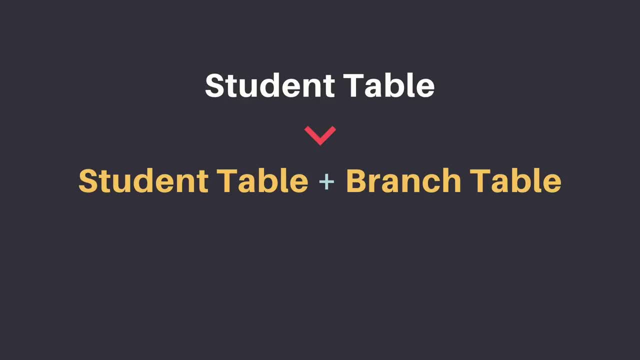 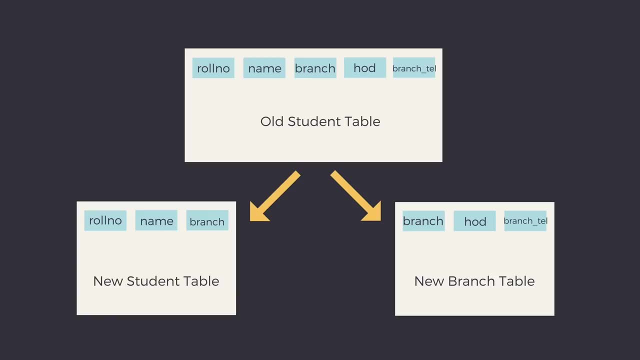 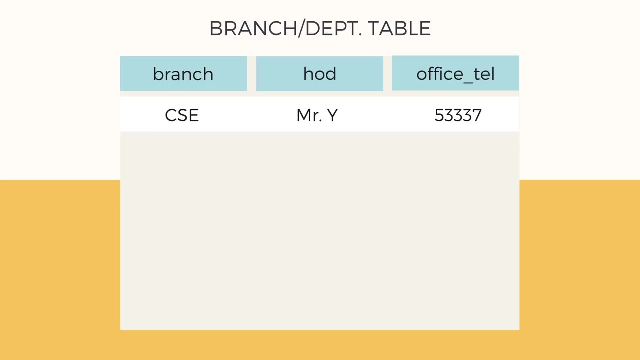 existing student table into two different tables: student table and branch table. the student table will save the data of student and the branch table will save the branch information. now, the branch information: if we want to save data of Computer Science Department students will be just one row that will. 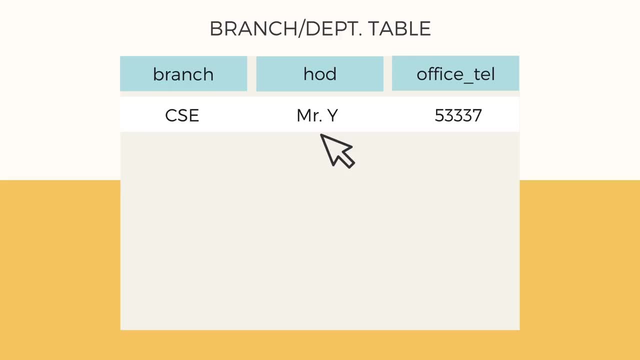 be the branch name- computer science- the name of the HOD- the new HOD, I must say, because the old HOD left- and the phone number of the department. and in the student table we'll keep all the information of the students enrolled for this particular branch and these tables will be related. 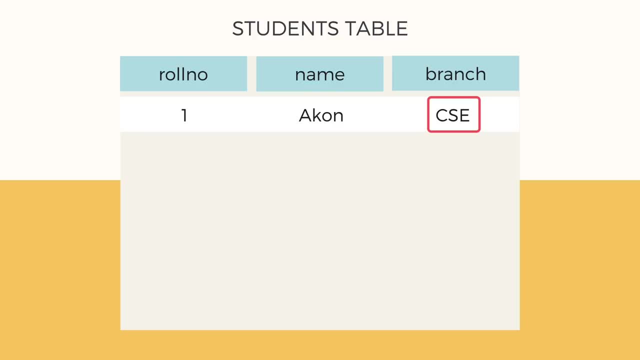 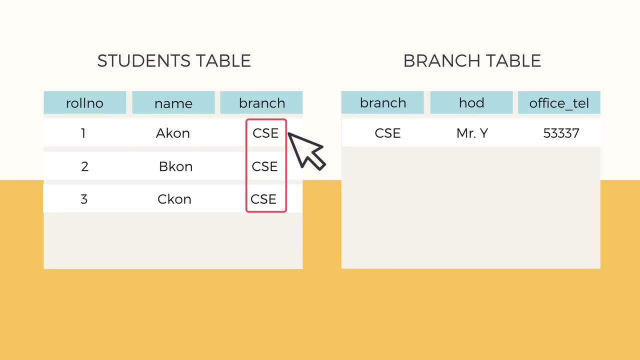 by the name of the branch. in our case, which is CSE, one can say that the branch name is still getting repeated in the students table. so normalization is not about eliminating data redundancy, it's about minimizing data redundancy. so now earlier, where all the branch information was getting,